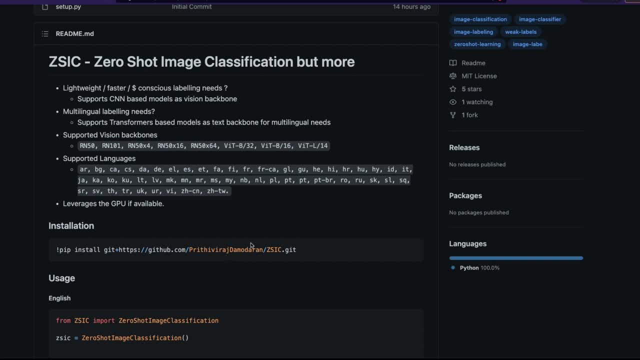 Thanks to Prithviraj Damodaran, who is a prolific open source contributor. I've covered a couple of his libraries already on this channel. So he has recently come out with ZSIC: zero shot image classification. And, as he says, zero shot image classification. 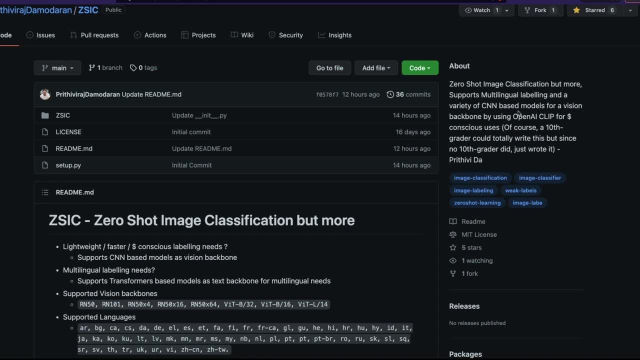 but more supports multilingual labeling and a variety of CNN models for a vision backbone by using open AI clip for conscious use cases. And there is a dollar in it And the main thing that I actually like this, of course, a 10th grader could totally write this. 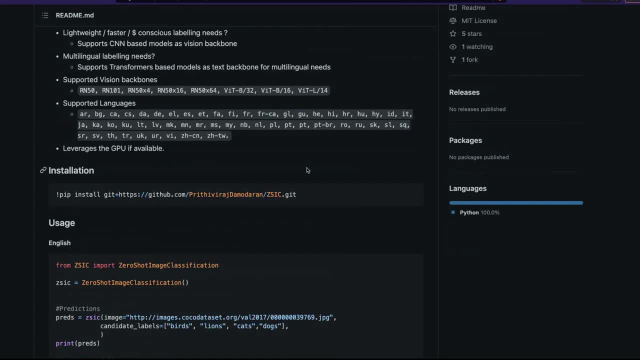 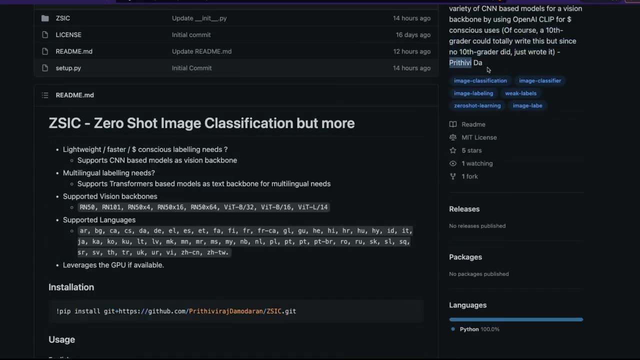 But since no 10th grader did, I just wrote this. This is amazing sense of humor, And also thanks to Prithviraj open source contribution. he he addresses himself, Prithvi da. So thanks to Prithvi da. 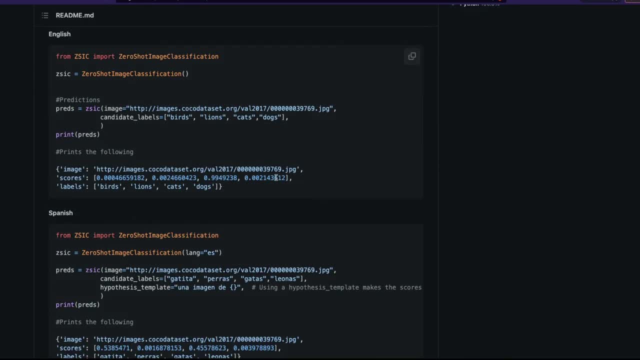 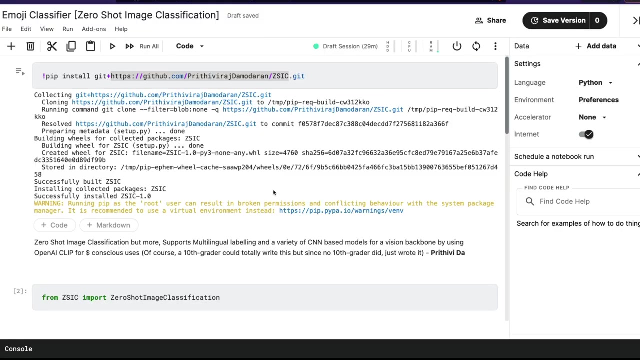 for for his open source contribution. we're going to use this library and do emoji classification. we're going to use zero shot image classification library z s ic for emoji classification And I'm going to use a Kaggle data set for that. The Kaggle data set and the Kaggle notebook and 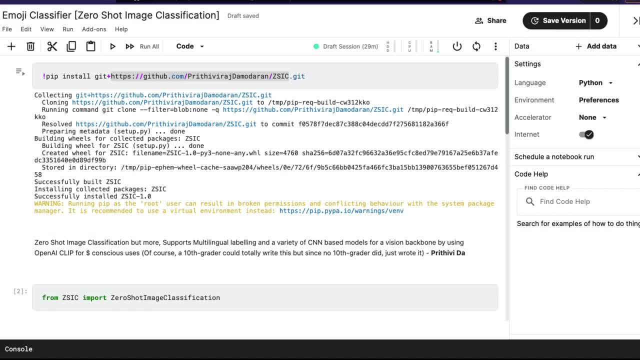 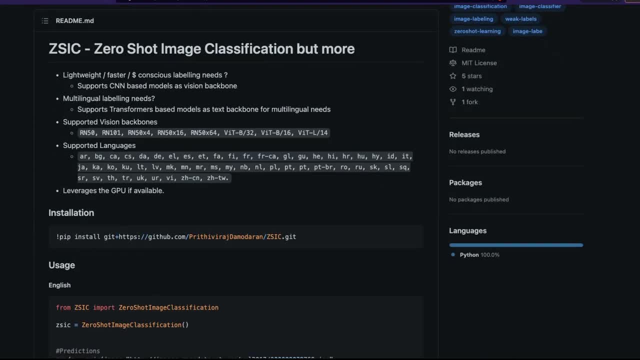 also the GitHub repository would be linked in the YouTube description. Please make sure that you start the repository and also give a shout out to the developer. This would mean a lot to the developer, who is also, you know, contributing to open source a lot. So now, starting with the Kaggle notebook, 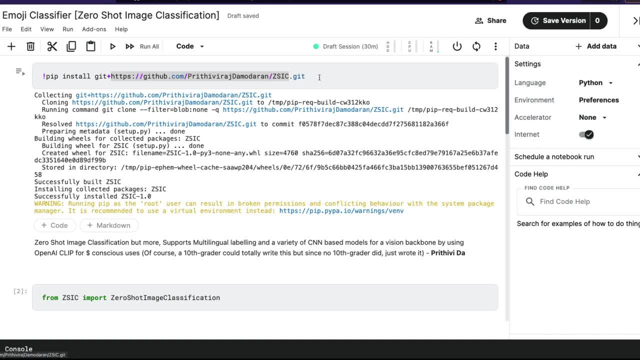 so I've gone to the Kaggle dataset page and then I've created a new notebook. the first step is to install the library. So, because it is- I don't think it is available on pi pi at this moment- So directly install it from Git. So when you install it from Git, 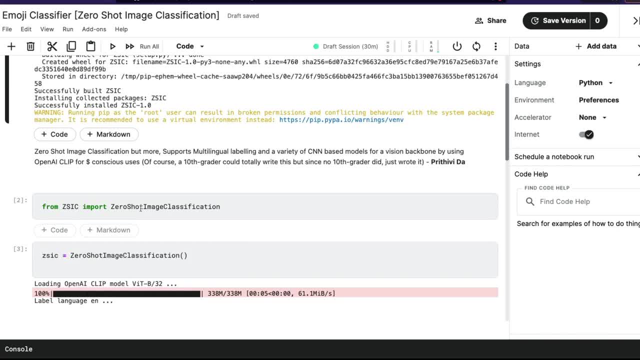 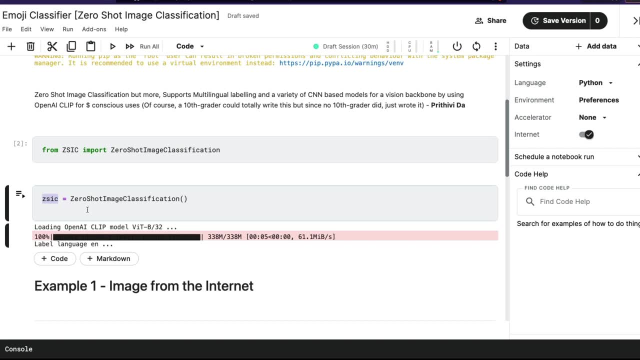 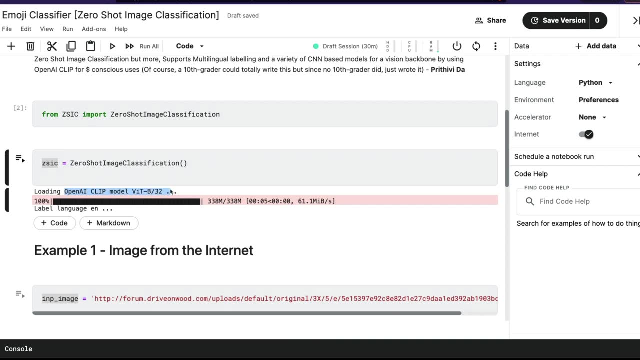 this is what happens, And after that you can import a class zero shot image classification from z s ic. After you do that, create an instance of z s ic like you can. you can do it whatever name you want And you can see that it starts loading the required model, In this case opening a clip. 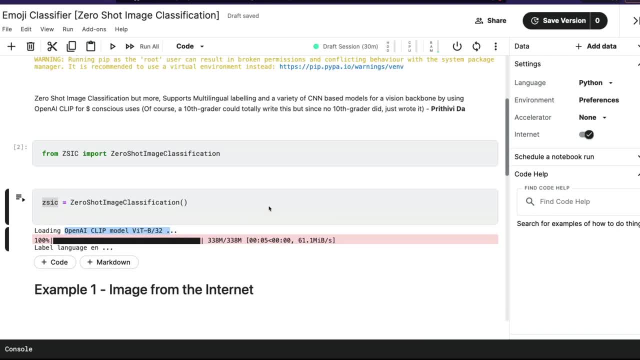 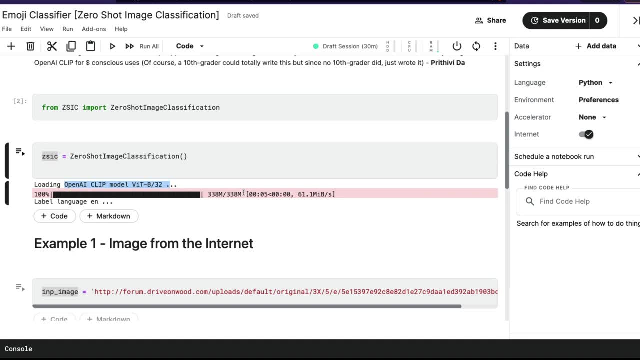 model with, with vit vision transformer. So at this point your model is ready. you have imported the required class, So which means you are ready to go do zero shot. image classification. Before we start with an emoji classifier, emoticon classifier, I wanted to show 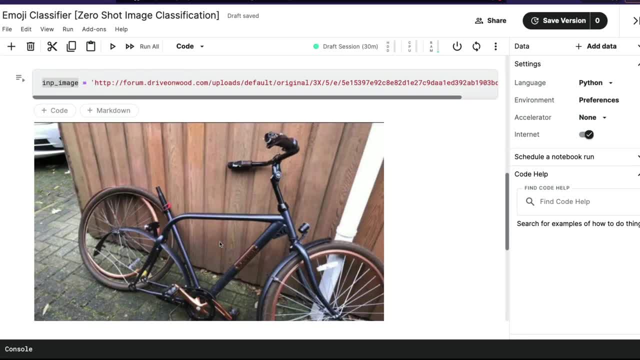 you whether it works or not. So let's go ahead and start with the emoji classifier. So let's go ahead and start with the emoji classifier, emoticon classifier. I wanted to show you whether it works or how it works first. The first thing is I've got an image from the internet which is a. 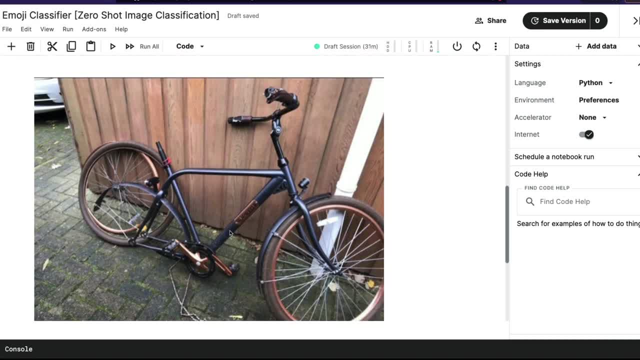 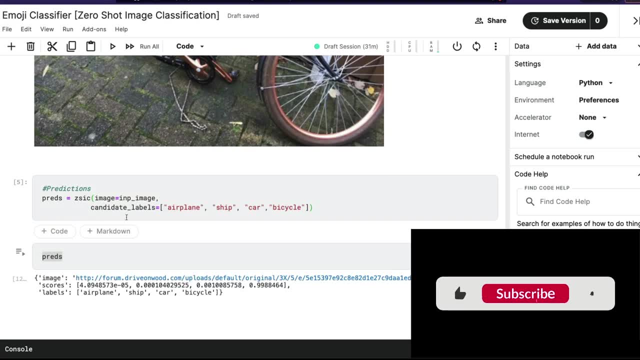 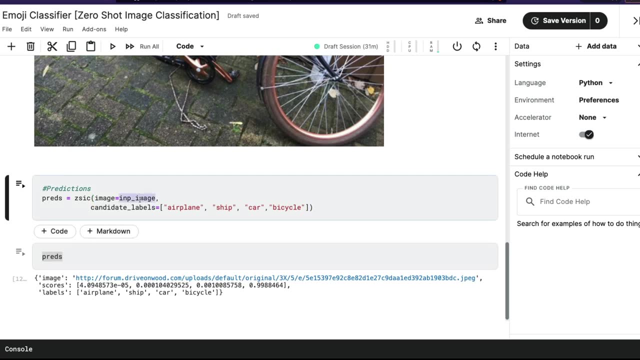 bicycle image. We all know this is a bicycle, But can we trust this model? So I'm going to ask this model: what is this? And the way we ask? a zero shot image classifier, very similar to the zero shot text classifier that's available with hugging face transformer. you pass on the input image. 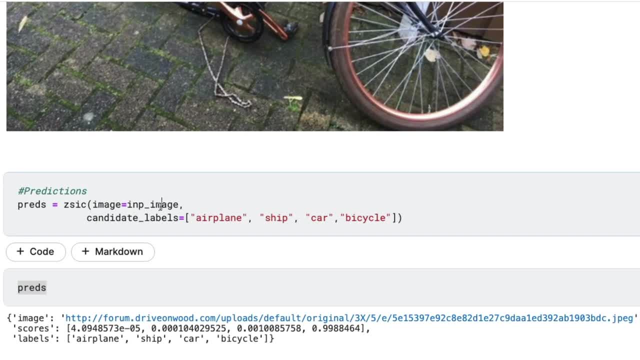 So this input image takes three kinds of attributes. One, you can give a URL that would download the image. from the URL to you can have a local file reference. but three: if you have got a pillow image, you can pass that pillow image. So you can do either of these three. right now I'm just passing. 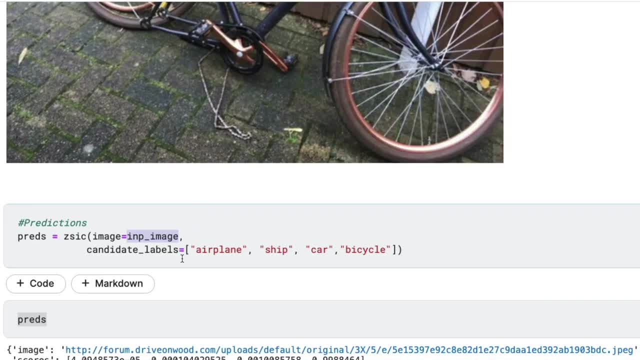 the URL. I've got the URL here. I'm passing the URL and I'm giving the candidate labels. So the candidate labels indicate or tell the zero shot image classifier that this image is associated with one of these labels, And then what is that label is what we are going. 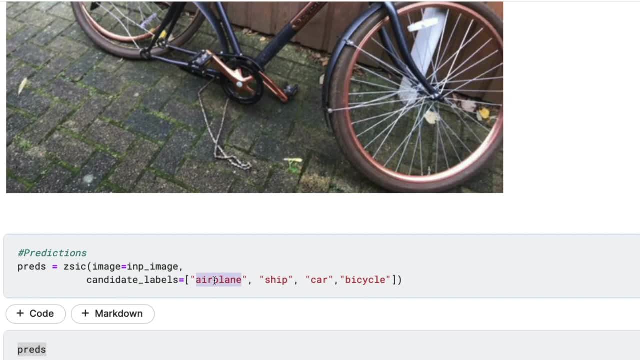 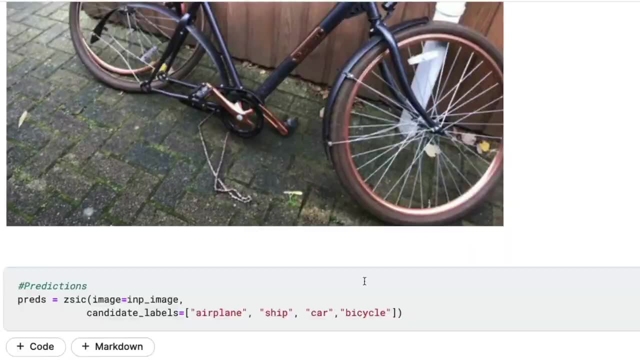 to figure out using the score that it gives. So I've given the candidate label saying airplane ship car bicycle. I don't know how does it look, But for me it looks like. it looks like a bicycle. But let's see what the image says, The model says. when I run this you can see that it. 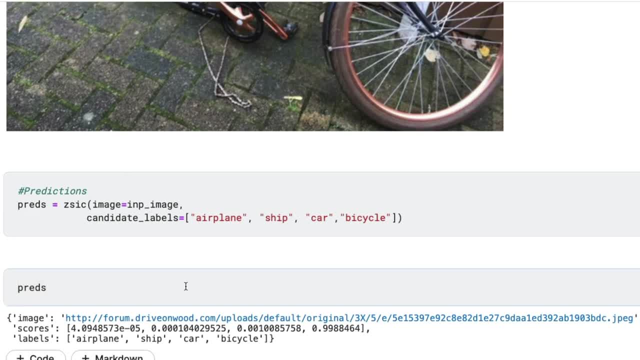 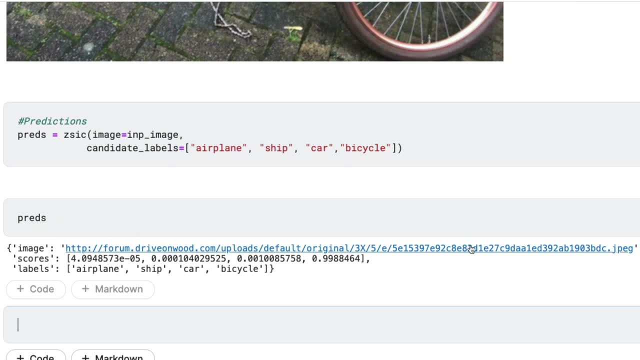 takes a couple of seconds, but it just finished. Then next thing is: when I print the image, you can see that it it has successfully managed. it has successfully managed to print the actual output, So you can see that it is a JSON object. you can see there is an image which says what is. 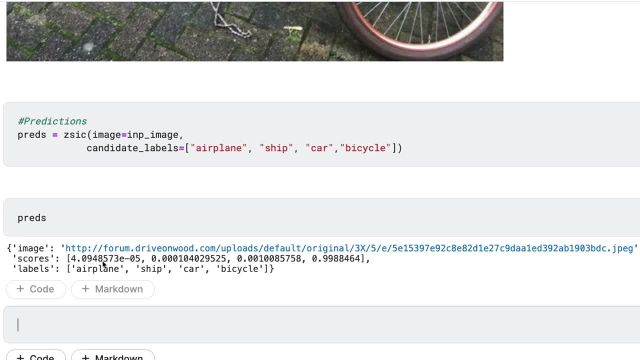 the input image, then the scores. you've got the scores and you can see the maximum score. if you see the maximum score- like for example if I do prints of score of max- you can see the maximum score or scores. 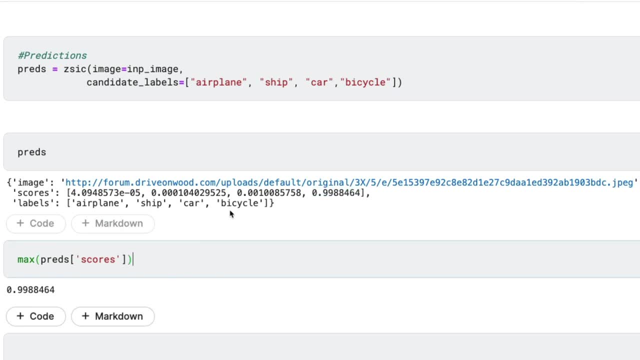 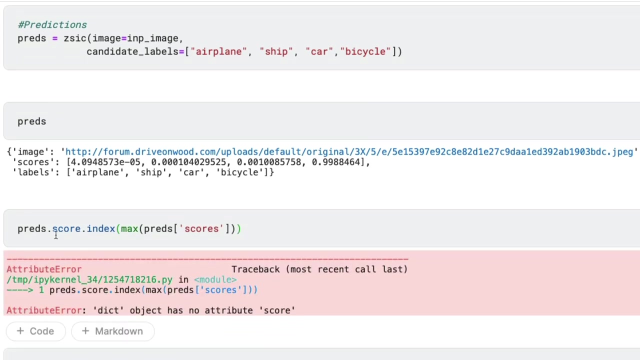 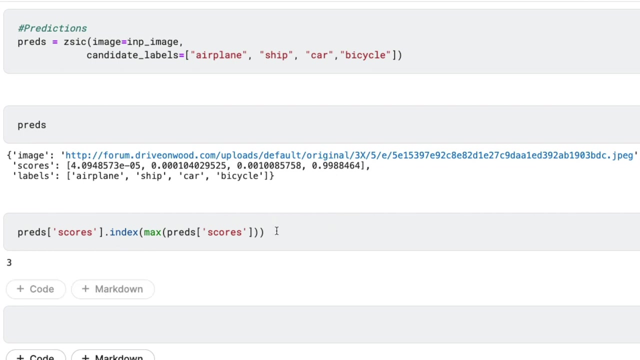 maximum scores is 99. And that is associated with bicycle. So you can basically see the prints of score dot index of, if I do that, oh, rates of score, scores of index dot index. that gives us the position where this maximum score is present. So now, at this point, you know the maximum score. 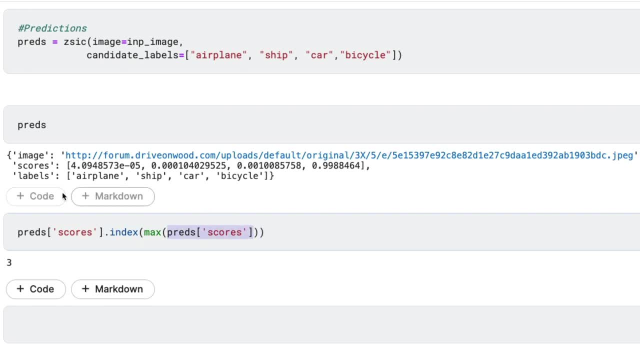 what is the maximum score. So let me print the maximum score first in a separate cell. So this is your maximum score. Okay, sorry, this is your maximum score And we are going to see the maximum scores label instead of manually printing. bicycle. I want to. I want to use this as a reference and 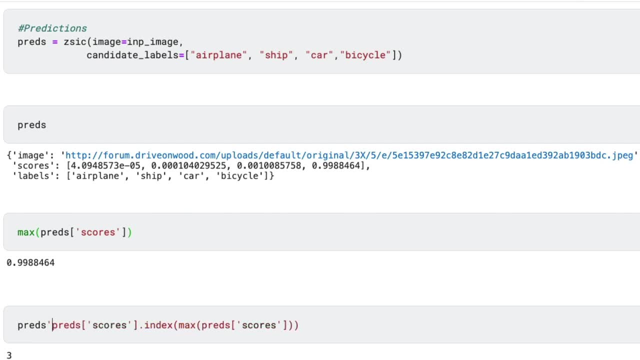 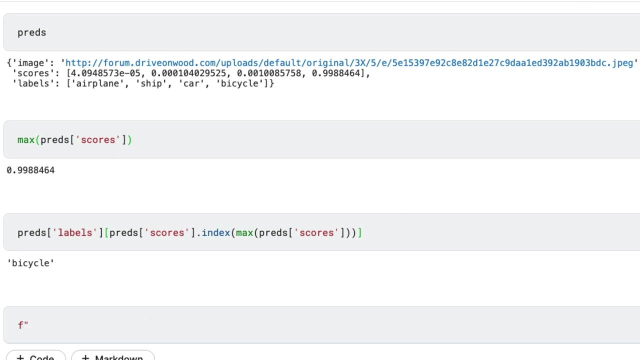 print it. So now I can say: prints of label, okay, prints of labels, labels And this as the index. now it would print bicycle. So now I'm going to put these things together in an F string, a very nice F string. I want to say f of what do we want to print? this image is a 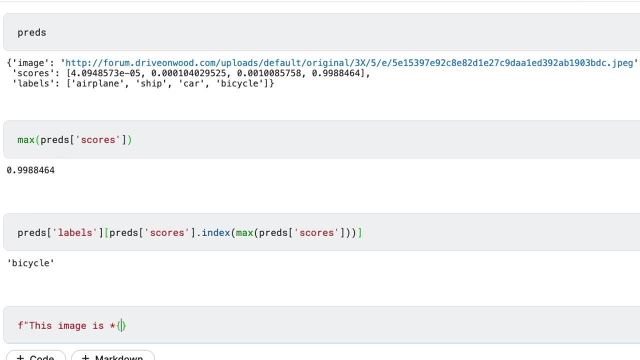 is, I should say, and then I'm going to put a star, I want to put this, this just close the string, and I'm going to write this with a score of: and I'm going to write this. So this is basically as: 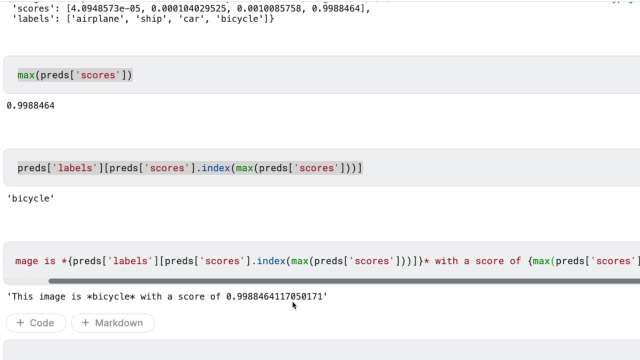 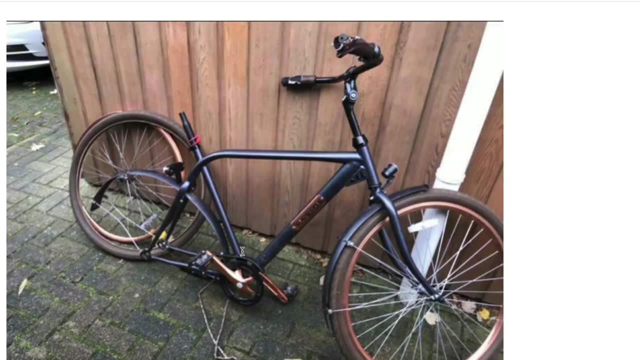 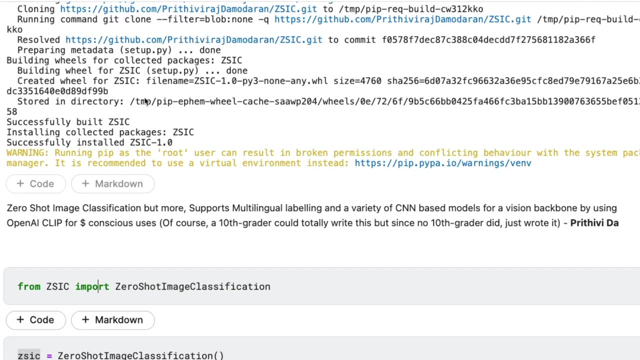 assuming that this image is a bicycle with a score of point 999.. So we have successfully managed to take an image from the internet. simple so the steps I would quickly repeat before we move on to the emoji classification. first, install the library. very simple, install it. 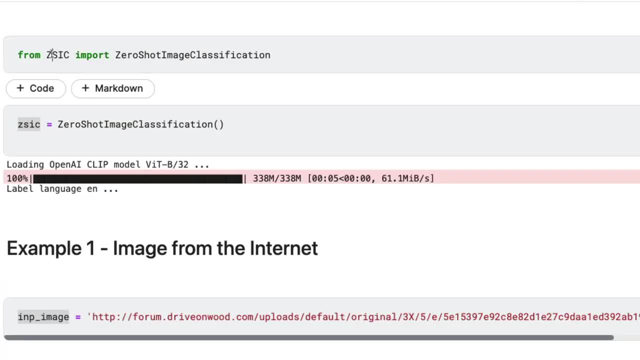 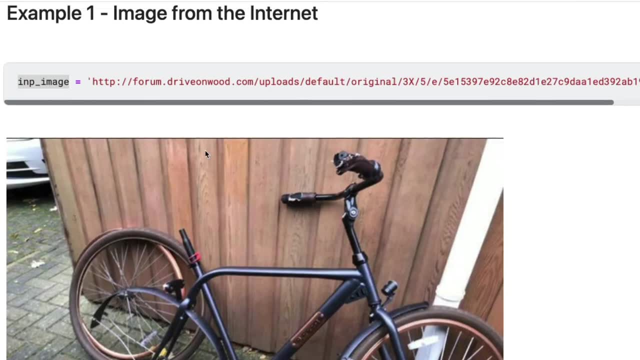 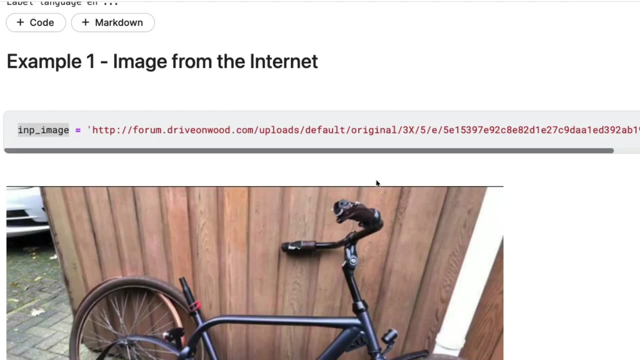 from git. second, load the library from zsic. import zero shot image classification. create an instance of zero shot image classification. that would download the required models. you can see the size of the models- around 340 mbs- and it downloaded fast thanks to Kaggle. next, get an input image that you want to classify and then you have to define the candidate. 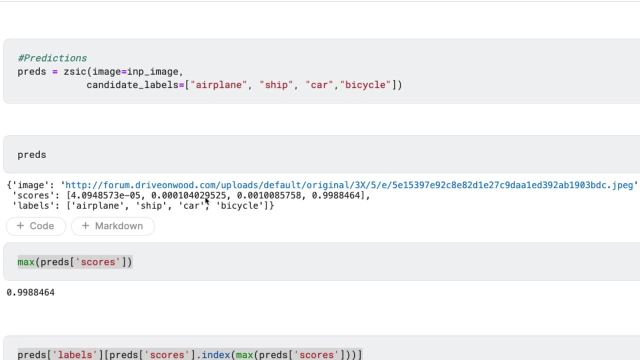 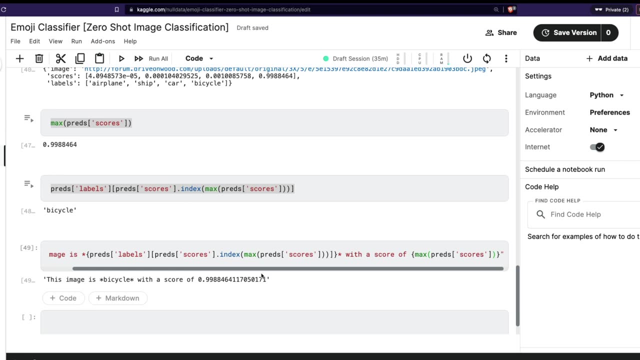 labels and then finally you have got. you have got the prediction, and then you are doing a little bit formatting to finally print it. so now I'm going to do the same thing for emoji classification. okay, so where do I have emojis? I've got a data set here and I've got 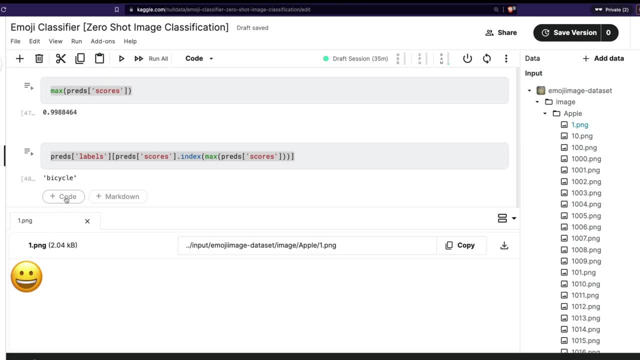 a lot of emojis and I can see the emojis as well here. so, but this time I'm going to do a little bit different, because I want to display the emoji as well, like I want to display the image. So what I'm going to do is I want to first call it emoji classification. emoji classification. 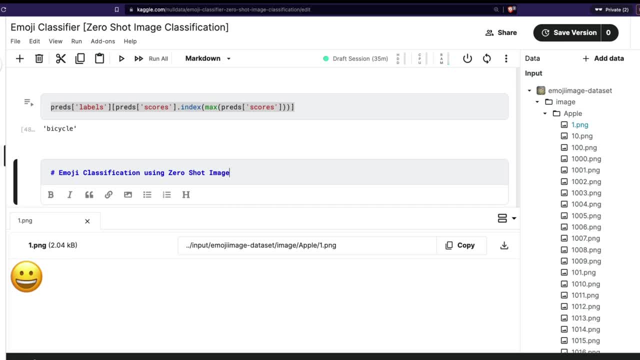 using zero shot image classifier. classification. classification is redundant, but that's okay. so now we have got the title. the next thing is we need to define the input image. so this is my input image. I'm going to copy this, but before that I'm going to load pillow from: 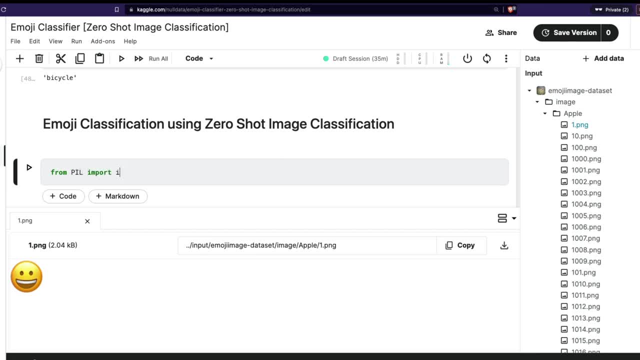 PL import image. Okay so, import image. so we have loaded image. the next thing is I'm going to open the image and store it inside an object. I'm going to call it in IMG image dot open and I'm going to give this. this is to show you that you can also give a pillow image object and also. 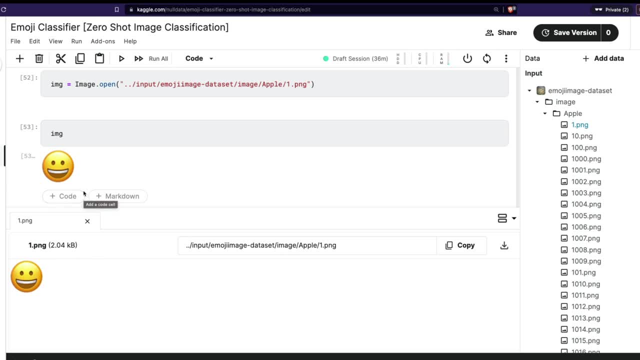 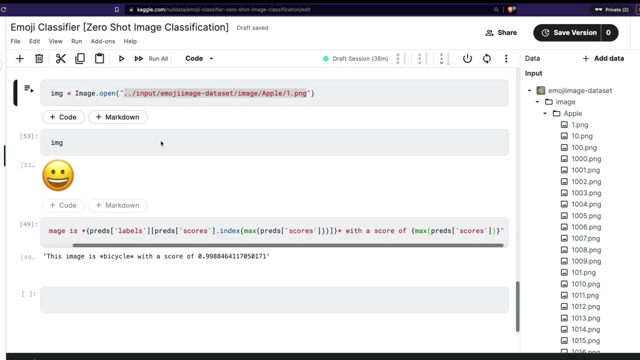 you can display the image like this, like I've got two reasons why I'm doing this this way, or you can directly give the local the local path, but I wouldn't be able to show you what image I'm using. So that's, that's the reason. so this, this one, I've got to move. I've got to move up. yeah. 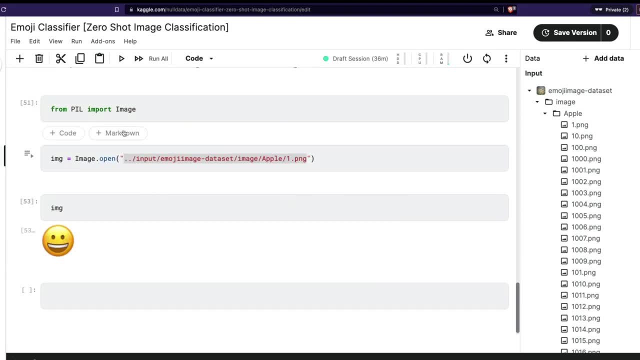 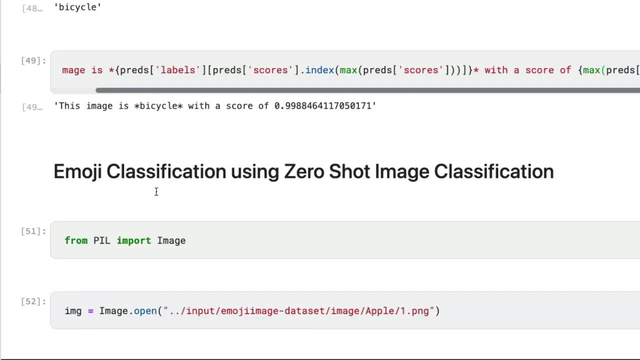 that you'll be there. you'll be there, you'll be there. yeah, we're good. so we have got, we have got pillow. we have got the input image, we have got the image. so I'm going to copy this from here, which is, we're going to do the predictions. so, predictions, input image. 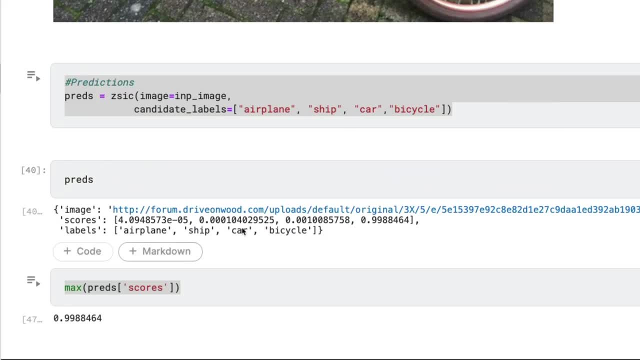 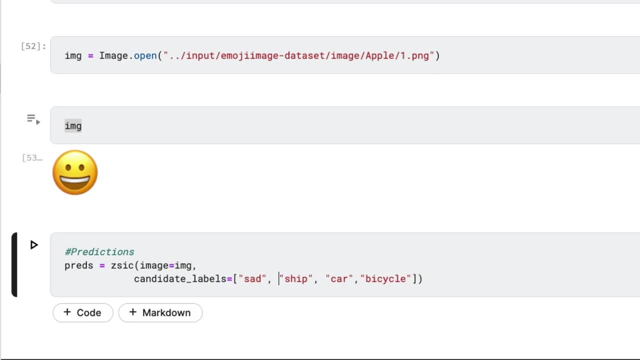 instead of input image, I'm going to give image. just the differences there. we gave a URL, but right now we are giving a pillow object. And what are the candidate labels? I want to say this is sad, this is anger, this is maybe, maybe crying, maybe ghost, I don't know. and finally, maybe happy. okay, I'm going to give. 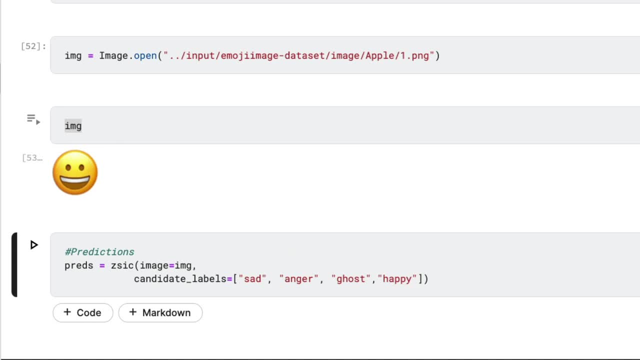 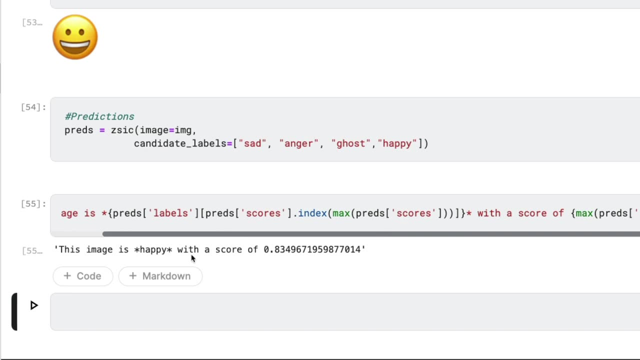 all these four options and I'm going to ask the classifier to classify the image. after I do that, I'm just going to copy this final that we just formatted and created and then going to paste it here and then you can see it says: this image is happy. 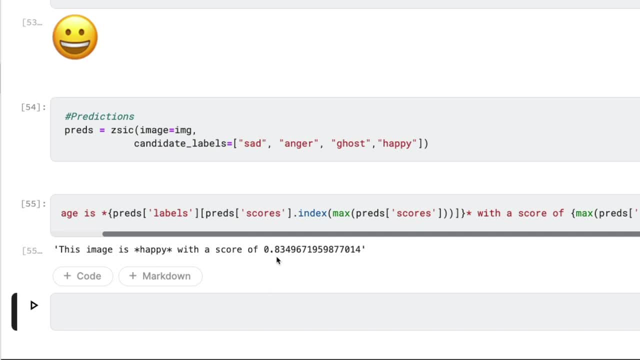 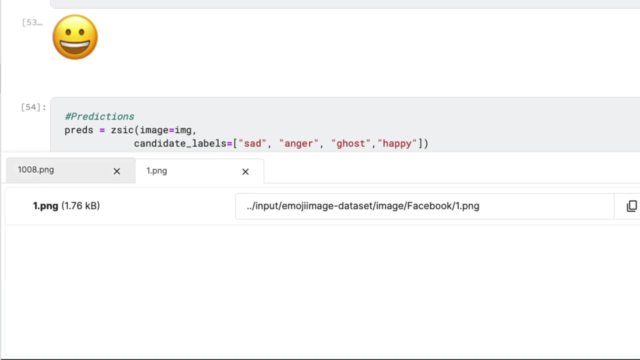 With a score of 0.83.. So you can see that this emoticon or this emoji, has been classified successfully using a zero shot image classifier. Let's try one or two more for us to maybe. maybe we can use a different, different one. 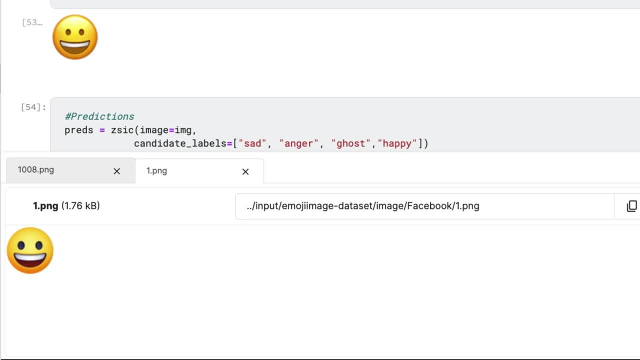 So this is Google. If I use- Sorry, that's Facebook, right. If I use Google one, how does it look? Do I have a different image? I've got an image, I think the finding the image. Okay, I think this looks like a middle. 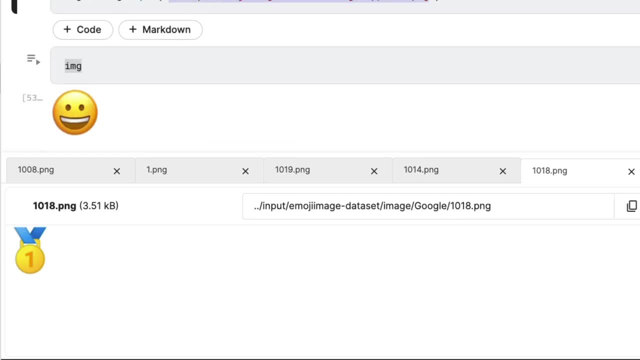 Let's see. Let's see if it works. I'm going to give this image now here. okay, I'm going to use this. This is my image And the candidate labels that I want to give sad anger first, and I'm going to say second: 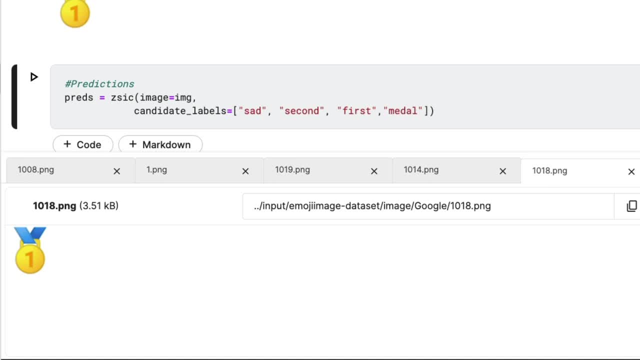 And I'm going to say middle, Let's see. Let's see what happens. Now, you know we are actually confusing the zero shot image classifier because it's it's both first and it's a medal. But let's see what happens. 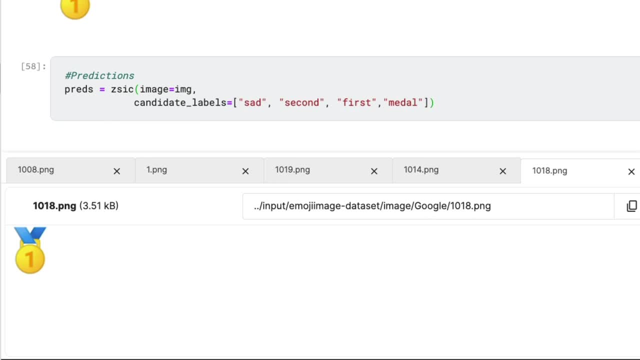 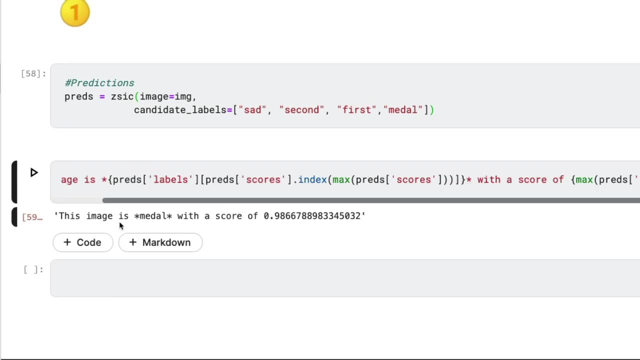 I'm going to run this and I'm going to run the next one to see what is happening. Let me close all these. Let me close all these images And then you can see. it says: this image is a medal with a score of point nine eight. 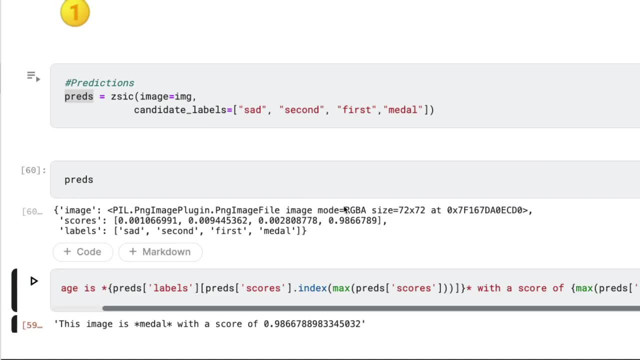 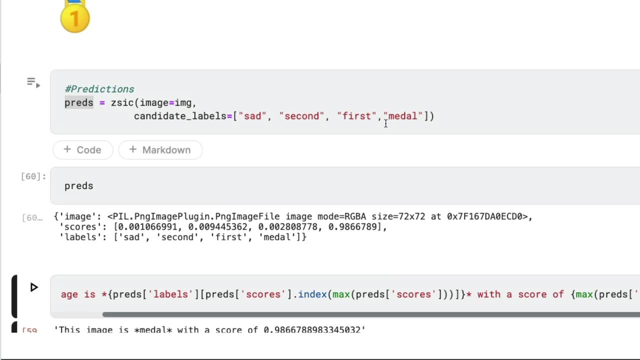 That's great, But let's, let's see the plates and then see what's happening. So it has kind of given point zero two for the first one, but it's still managed to classify this as middle. So now what happens, Let me. I wanted to try one more thing. 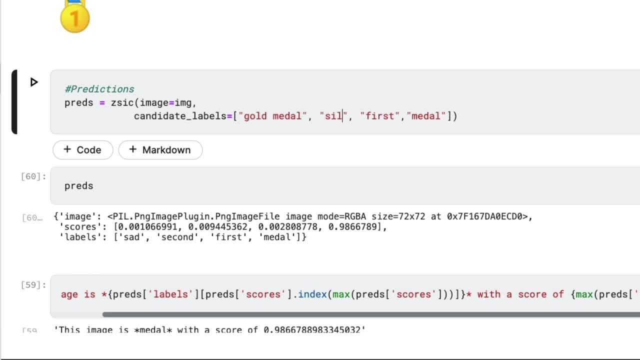 Here I can say gold medal, I can say silver medal and I can say a bronze medal. okay, and I don't want to give the fourth one is fine. So now I'm going to do the same thing, But instead of just generically saying medal, I want to check whether it is a gold medal. 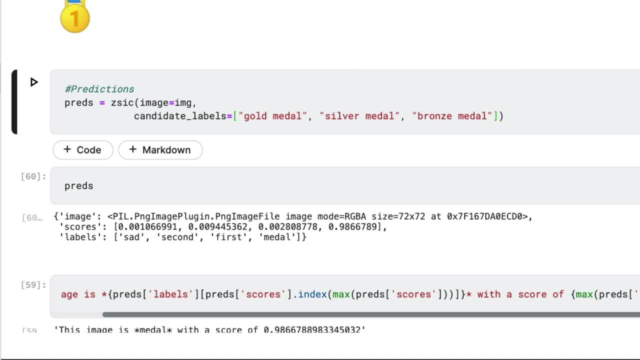 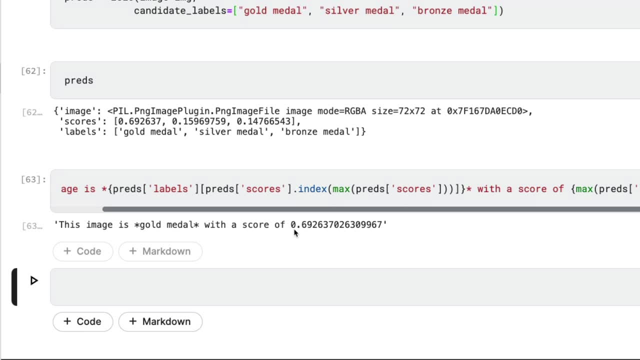 silver medal, bronze medal: Again, I'm just trying it out. I'm not sure if it's going to give the result that we want, using zero shot image classifier printing out the parade, but that's not important. It says it's a gold medal with a score of point 6926.. 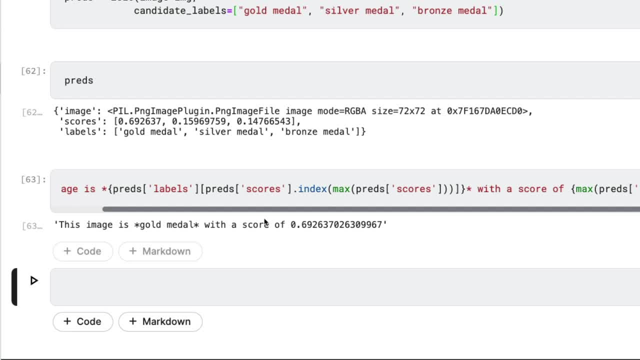 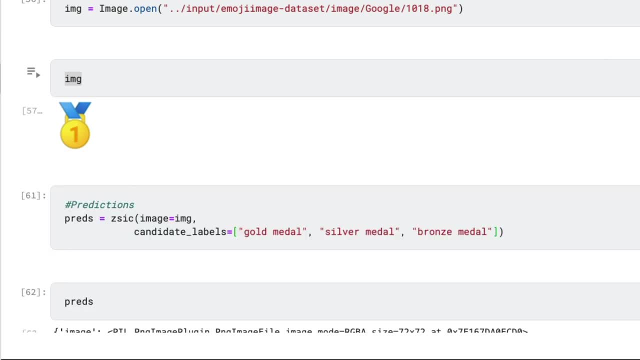 Where did we find it? Where did we find the silver medal? I want to take the silver medal now. What is the name of this image? It's point nine eight, right, So let me take the silver medal. I'm going to take the silver medal, which is 1019.. 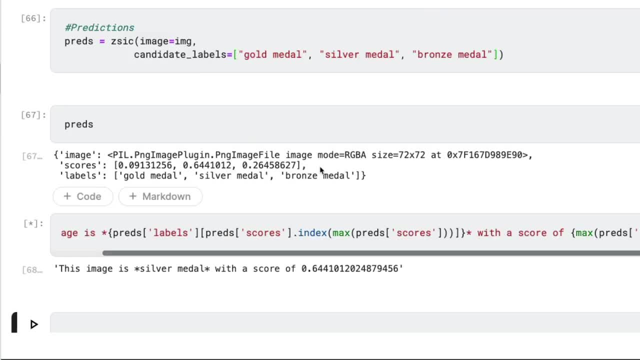 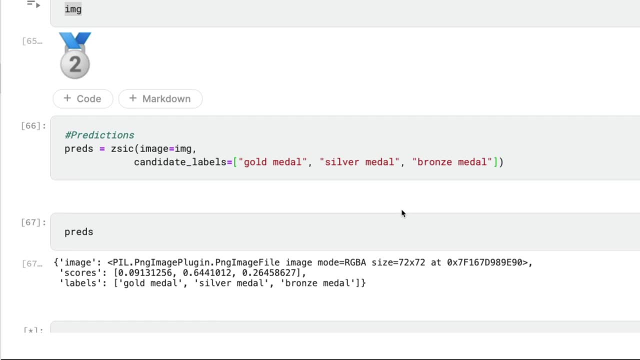 And I've got the silver medal. let me check what happens. Oh, it has successfully classified this as a silver medal. That is amazing. I don't know if these things were part of the training data set. I'm not sure. I'm not sure how clip has been trained, all those things. 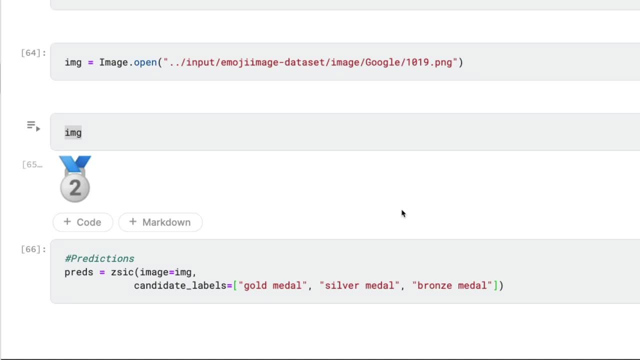 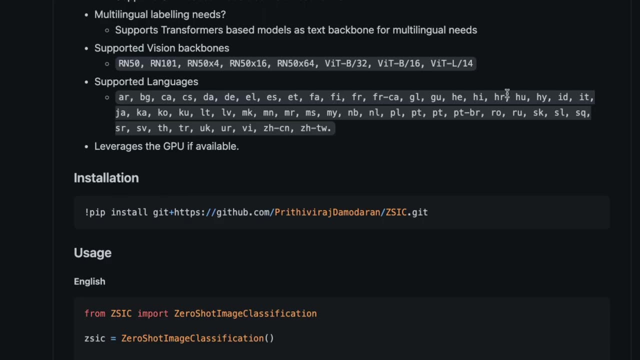 But you can. you can actually see that it is doing a great job, Even though it is a silver medal. It's a zero shot classifier, And the greatest thing about the zero shot classifier that Prithviraj has built is it's not just for English. 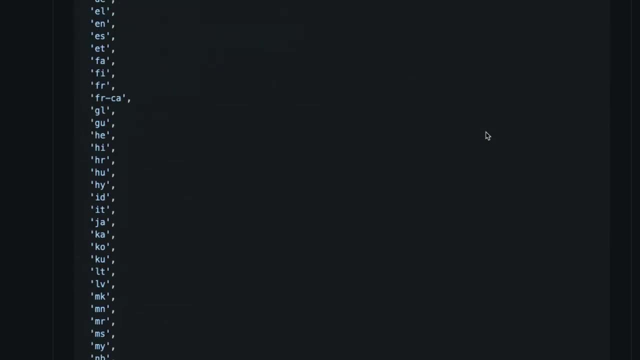 It's not like it works only in English. It supports a lot of languages. you can see all the languages that it supports. I don't know most of these languages, So that's why I'm not using it with any other language, But you can see it supports most of these languages. 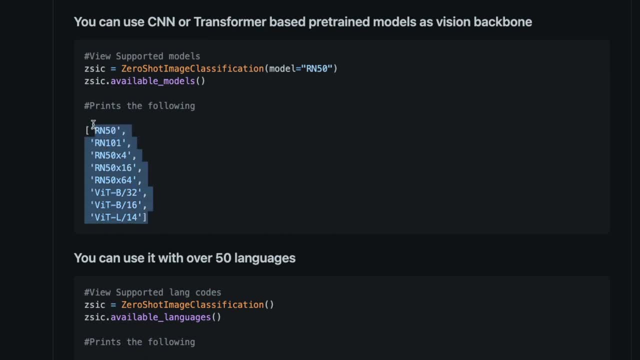 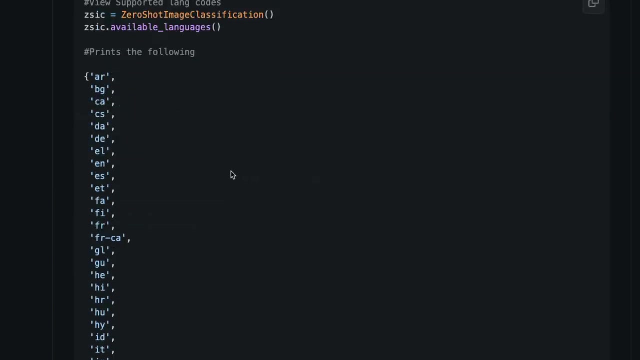 And the next thing is not just the multiple languages, you can also attach multiple back end. So right now, by default- I think it uses a wit, but you can, you can, you can you see in a transformer based model for vision back backbone. so you can, you can do one customization. 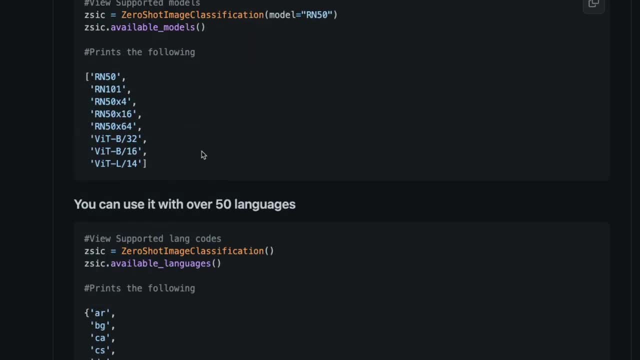 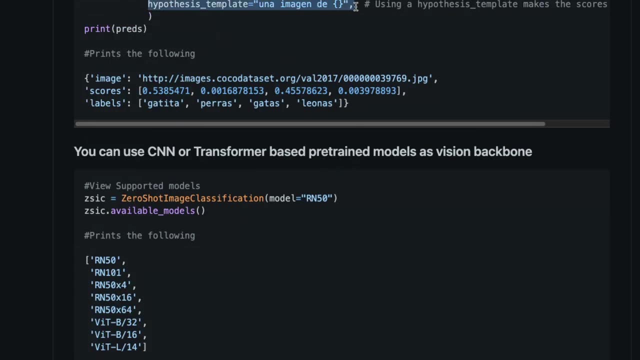 you can change the language to, you can change the backbone for for the vision, backbone Three, the entire thing that you see here works based on the hypothesis template. So if you see the note on the GitHub repository, by default for English the hypothesis template. 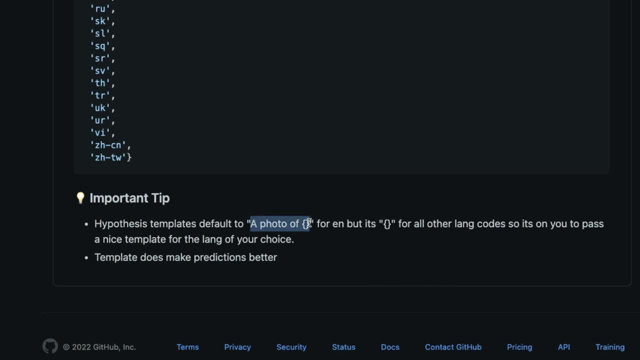 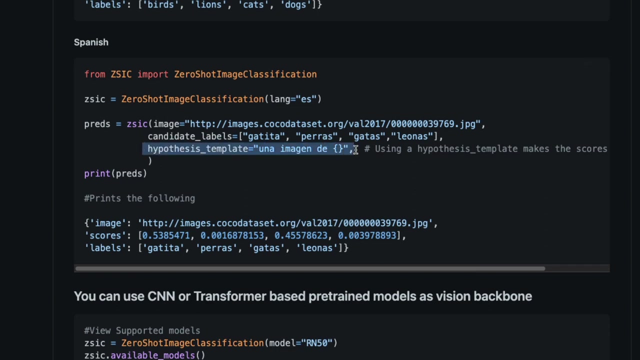 goes like this, But for different languages. it is defaulted to this, which means there is just a parenthesis. So if you want to improve your result for different languages, then you need to manually give a hypothesis template. you need to give a hypothesis template as one of the arguments. 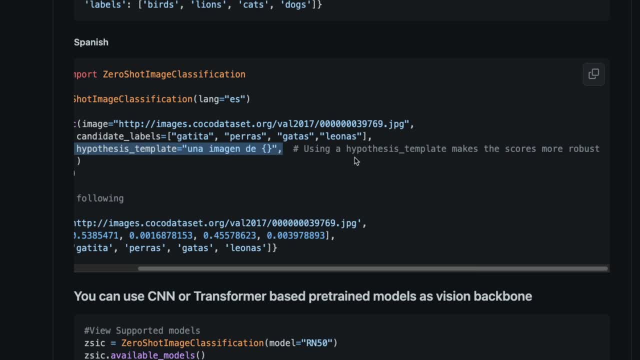 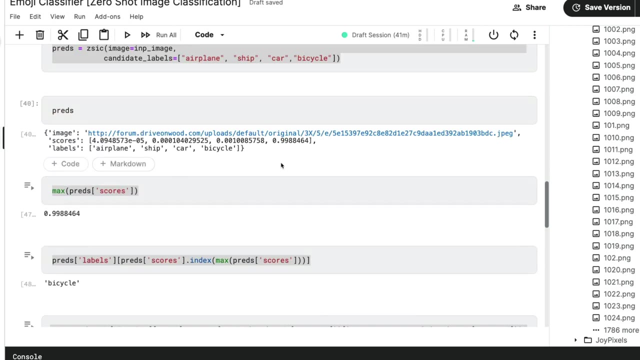 that helps the vision classifier, that helps the zero shot classifier to make robust predictions, course, because it tries to. so what it basically tries to do is that text that you give this photo is off. that's what it tries to align with each of these object and then whichever. 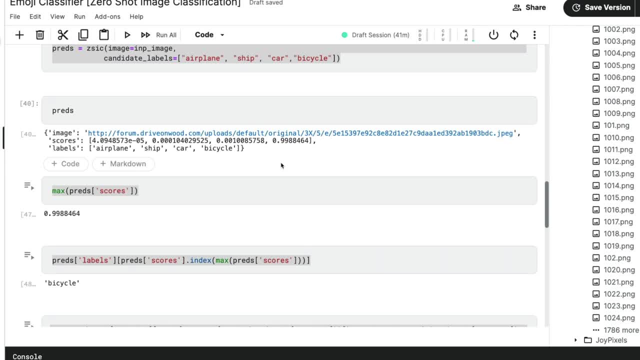 is closest, then it will try to give you the appropriate score. So by basically optimizing the hypothesis template, you can improve the scores that you're getting. you can, you can optimize the results. So overall, this is an amazing, amazing library. just like I say, like, make sure that you go. 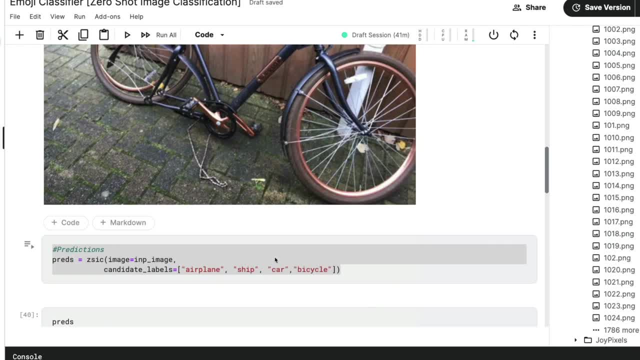 give a star to the repository and then and then give a shout out to the developer. But so far we have seen that it works very well with emoji classifier and auto classifier. So that's it, Thank you, Bye Peace, Also for any image from the internet.